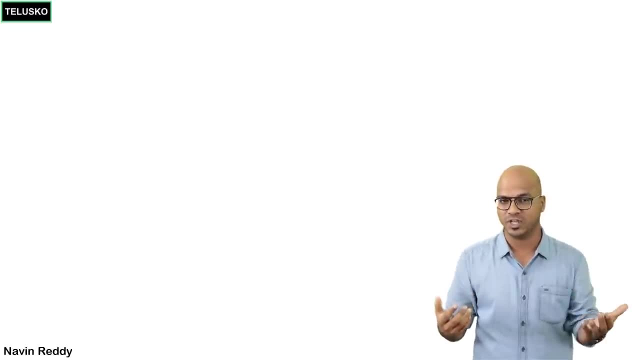 important. or maybe the showing of images, showing of videos, are very important. So you can, you know you can- take all those things are important requirements. Then you can have the site to prioritize them. So that's one thing right. First of all, you have to create requirements and 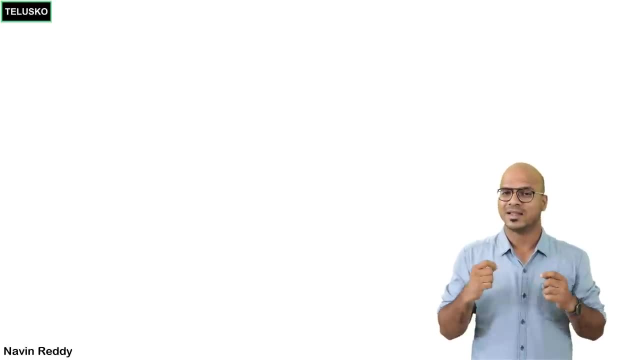 then you will start working on the requirements. But if you are following Scrum, Scrum normally goes with sprint. Now what is sprint? So let's say the entire project might take one year, but of course you will not be waiting for the entire year to deliver the product. Of course your client will. 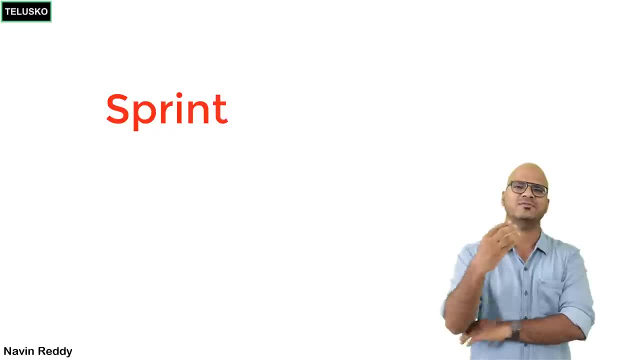 not be waiting for you to deliver product in one year. So what if you can give something to your client every two weeks, or maybe one week, depending upon your speed? So maybe after every week or two weeks or four weeks, you will deliver a product. Now this can be a potential. 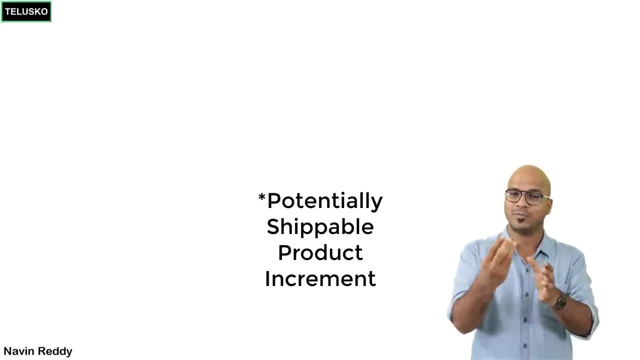 deployable product, but not every deployment or every product which you give to your client after four weeks will be deployed, But it is potentially So. if clients want to deploy it, it's their choice, right? So if you want to do that, what you will do is from the entire product requirement you have. 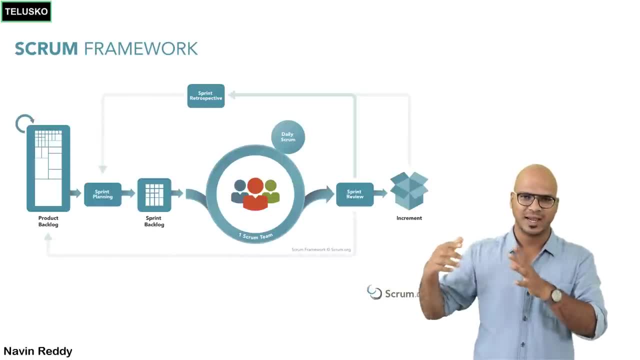 you will take some requirements for each week, right, So to understand that. so we have the first one here, which is which we normally called as a product backlog. So we have the entire backlog here, which will have all the requirements from start to end. You can add the requirement later. 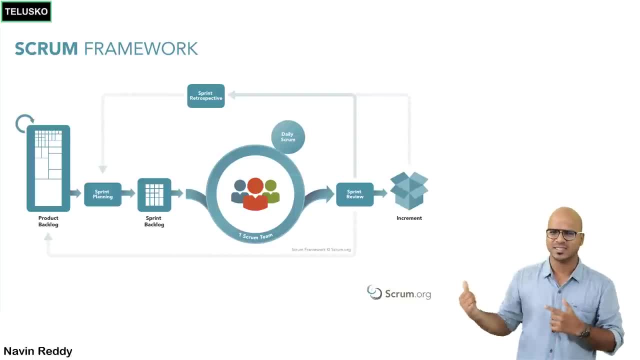 as well. okay, So let's say we have a big requirement you have. you can break it down for the current sprint or for the current week, Other requirements, you can just have it as it is. You don't know how to work on it- or? 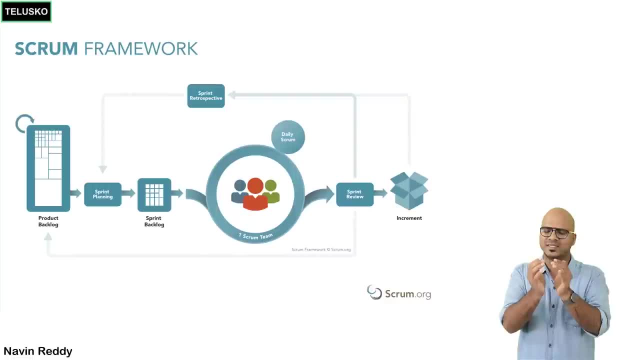 what are the sub parts of it? We can define them later, right, But let's say, if you have a module with you or if you have a set of requirements with you which you can complete in one or two weeks or four weeks, Now that will define your sprint time. So one sprint is one week. So if you 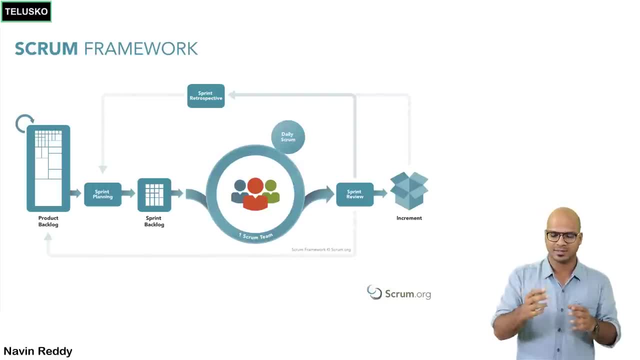 define for two weeks. that's your first sprint. you will take some requirements from the backlog right And you will call the current sprint backlog. So for two weeks right Now it will, of course it will have a less number of requirements, But before that you have to also plan your sprint. 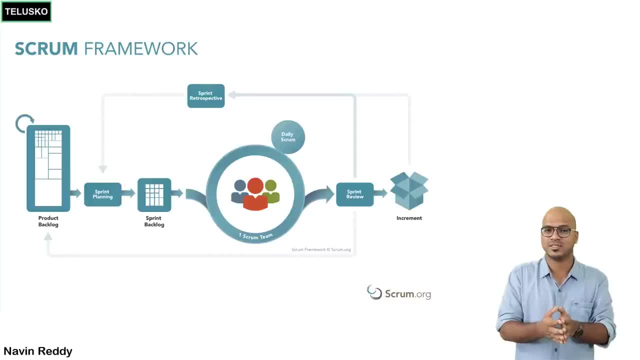 right What you will take and then what are the requirements we have for this. So, basically, we got a product backlog, then you have to plan and then you will get a sprint backlog. Now, once you have a sprint backlog with you, and now you have two weeks, let's say this is Monday and for next two, 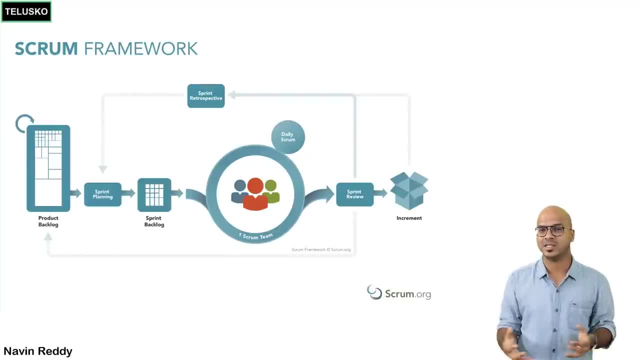 weeks you have to work on this product. So what you will do now? you will start building the product, but who will build it? Of course, we'll talk about roles, but basically we have a scrum team. Now, if you, if you are thinking we'll be having a big team or not, exactly because we have talked about that, 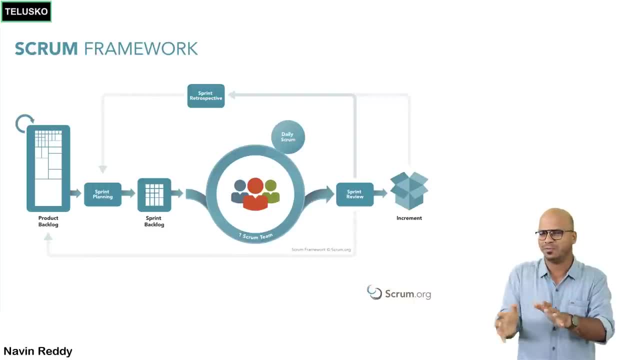 in Agile, right, You need a small team, maybe around four to eight people max, right? So on average we go for six to seven people, right, That's the average we have. So let's say, you have a team with you Now. this team will work on the product and after the first sprint, let's say after two weeks, 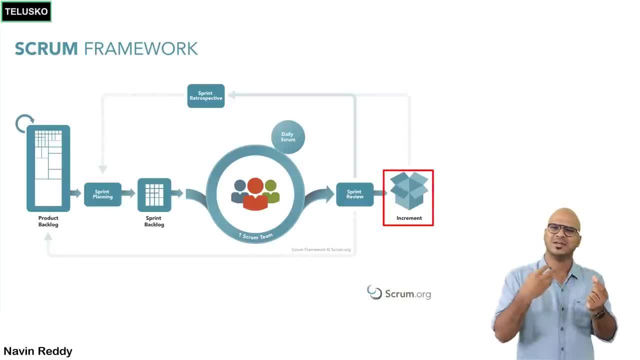 increment. So what is the increment? you can imagine this as a potentially shippable product. okay, So let's say, if you are building Facebook, you've got a first page where you can post feeds or you can see feeds. that's your first increment. Now, this is not the actual Facebook which you 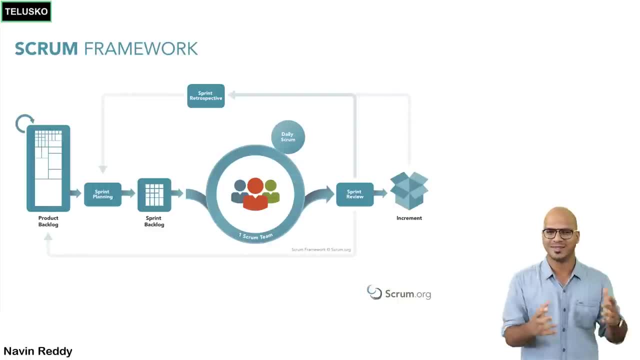 wanted. but you got something right. You can deploy the product on first two weeks, right. So that's the increment. But it may happen that in your first sprint you were not able to complete all this sprint backlog. Now what you will do? you will send the remaining backlog in the next sprint. Yes, that. 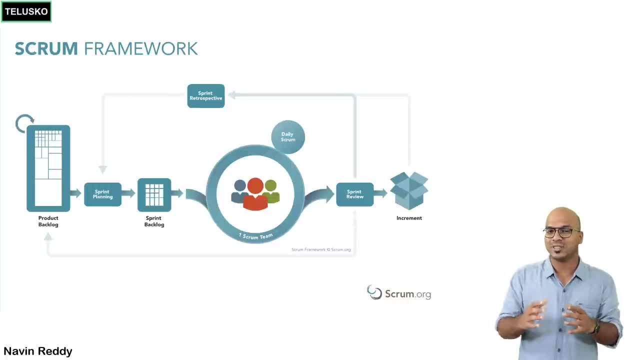 is possible. Okay, There is no hard and fast. Of course, in the next sprint you will complete the backlog from the last sprint and you will take some extra from the product backlog. right, Of course, you have to break it down, You have to. 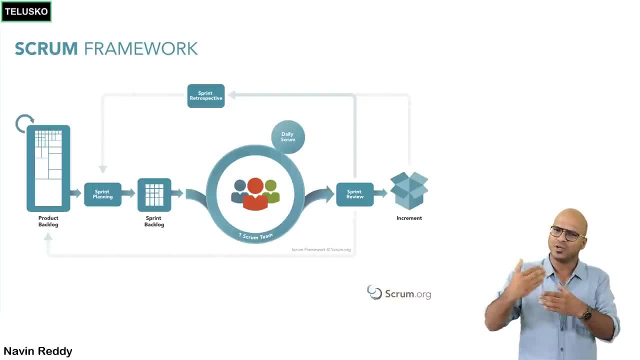 take in the current sprint, You have to plan first, right. But before even going for the next sprint, you have to do a sprint retrospective. Now, what is that? Now, think about this: When you are working on a product, let's say after you have completed two weeks, Now, in those two weeks, in that first, 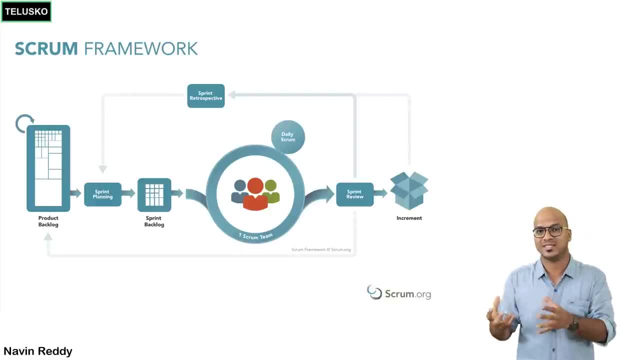 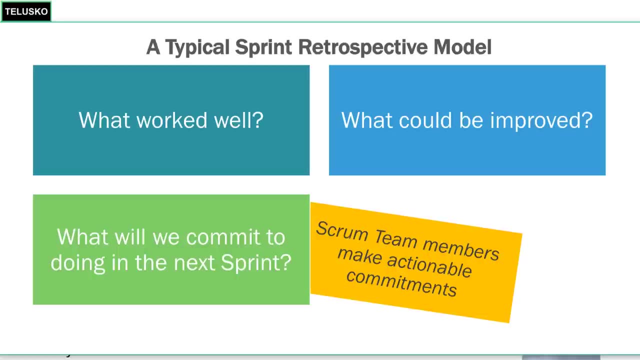 sprint. you understood something, You have learned something, You have you did something. well, This is what you do in the retrospective, So normally you talk about what worked well, You talk about what could be improved in the next sprint and then what will we commit to do in the next sprint? 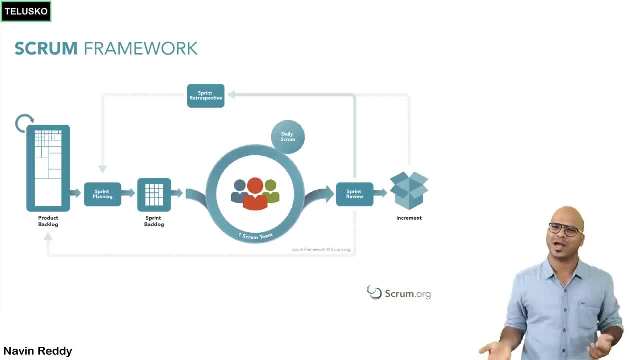 right, And then all the team members, they will have their own comments. So, in fact, when we used to work on scrum, so basically we used to take sticky notes and we used to write the comments, you know what? what went well, what is something we can do in the next, next sprint, So you can post. 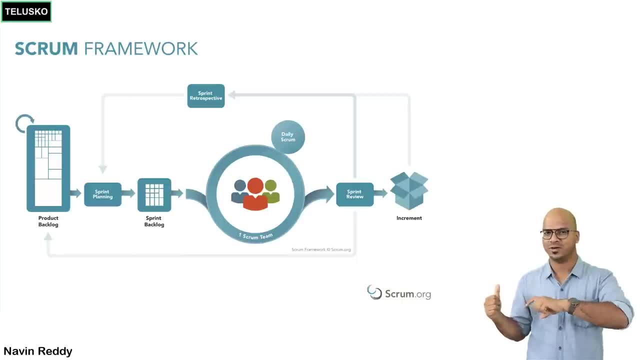 that on the board. So that is basically your scrum framework. So, if you talk about the events here, we have a sprint and then we have to do sprint planning. There will be a daily scrum and that's something we have missed. So every day, for 15 minutes, the team member will come together and 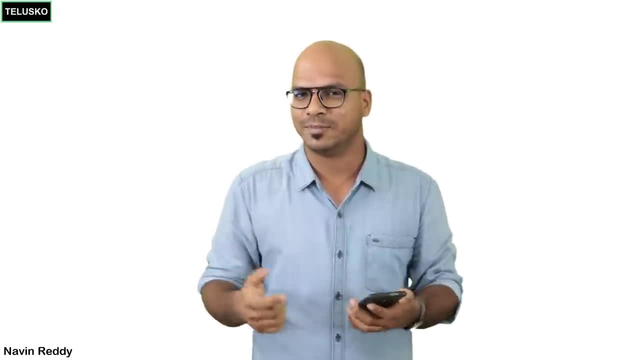 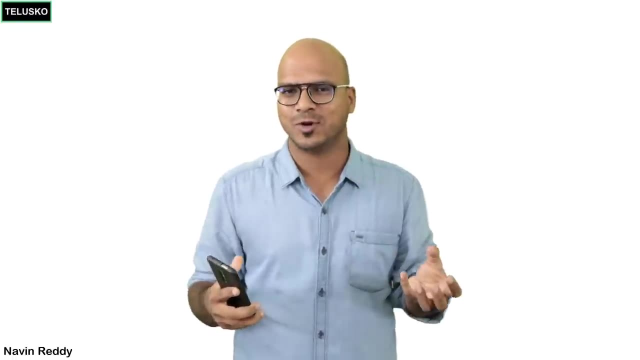 they will discuss. So this is basically a stand-up meetup. Why stand-up is because you don't have to waste your time discussing every aspect, because the moment you sit on a chair, your mind goes slow down and then you will talk about something else and then there will be a huge discussion. So to 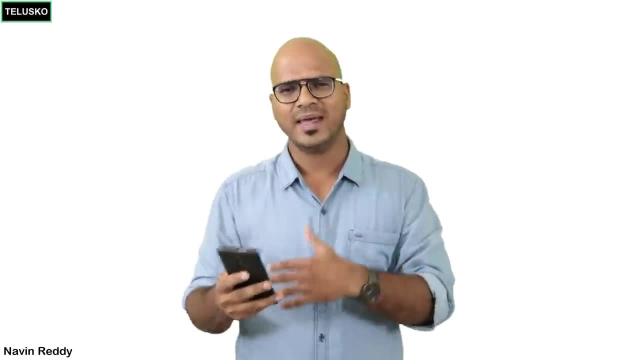 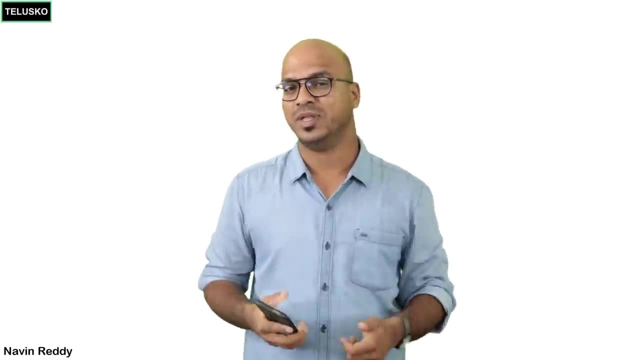 solve that. there will be a stand-up meetup for max to max 15 minutes and then we have a sprint. if you talk about this, what are documents you need or the artifacts you need? The first thing you need is product backlog. We have talked about that. this is the entire requirement you have. Then we have 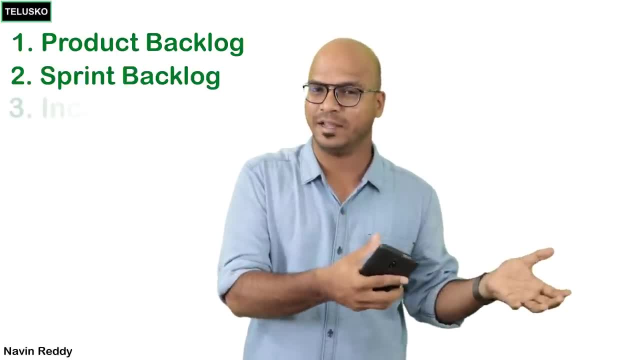 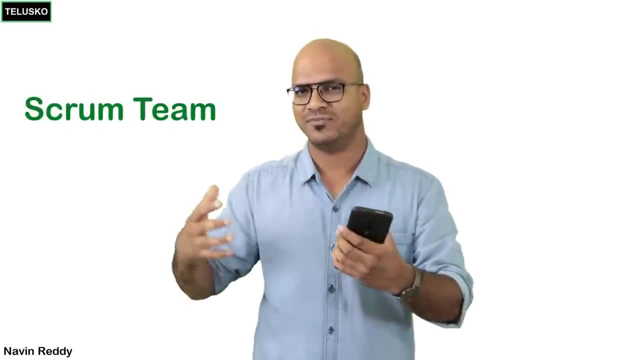 sprint backlog for the current sprint right, and then we have an increment, which is the shippable product. But we have one more question here: What are the roles of people here? Example: we have scrum team. of course the scrum team will have developers, testers. Apart from that, we have two more important. 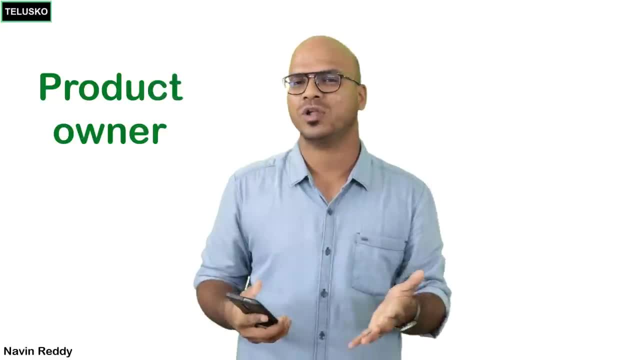 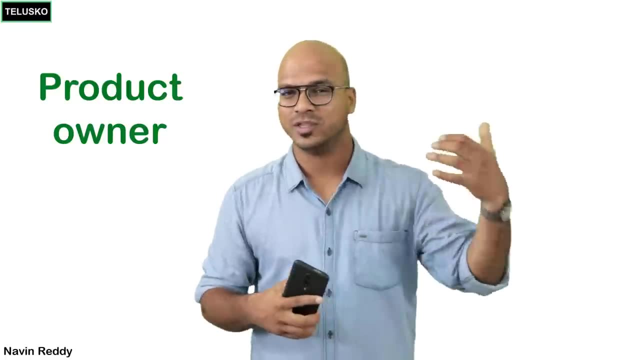 role here. The first one is the product owner. Now, who is the owner of the product? Of course not your client or the stakeholders, right? So a client will give all the requirements and you will get the requirements from the product owner. So the next one is very important- is scrum master. So who? 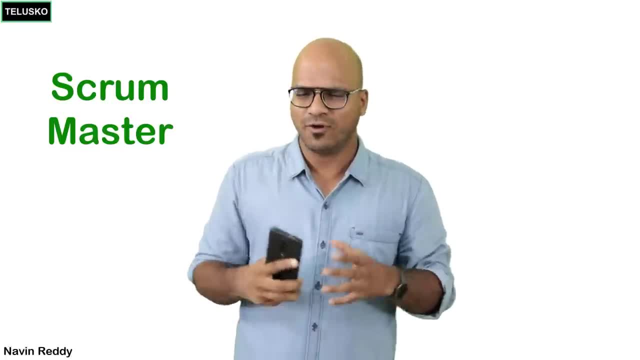 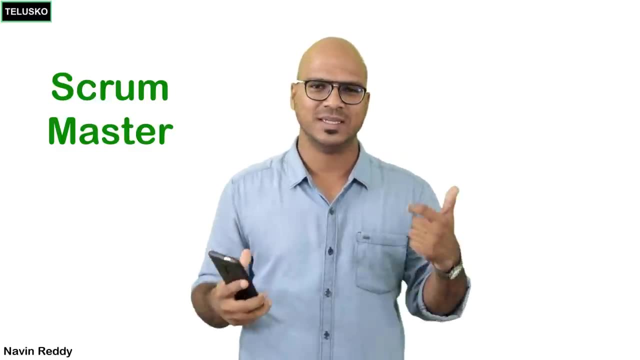 is responsible to manage the entire scrum working. Of course, our development team. you're focusing more on development work, So we need someone who will manage this scrum meetup. you know stand-up meets and then retrospective and helping people achieving tasks That can be done by scrum master. So what? 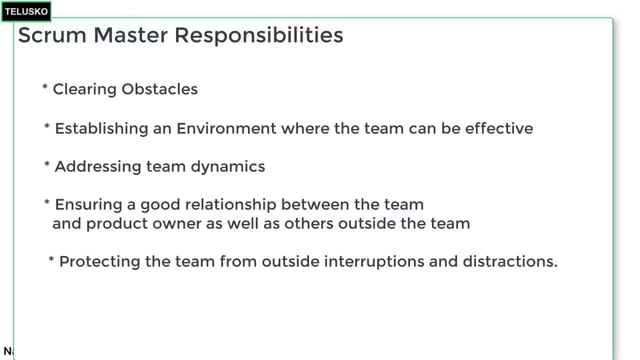 are the tasks of scrum master. So they will be clearing the obstacles, establishing an environment where the team can work effectively. So they will be also protecting the team from outside interruptions and distractions- and this happens a lot. right, As a developer, you want to focus on. 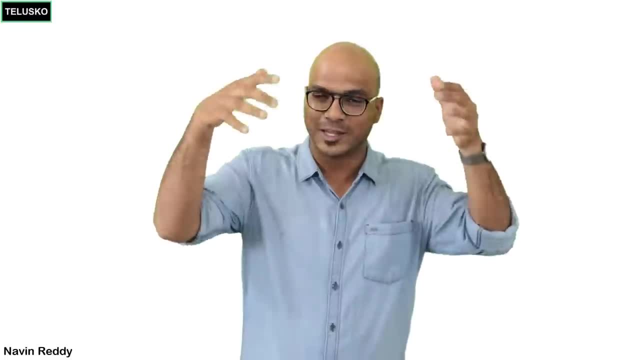 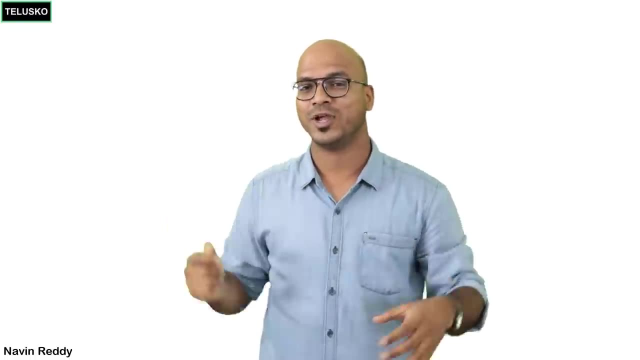 your work right and normally it takes around half an hour for the developer to get into that zone, right? So when you start working on the machine it takes at least half an hour to get into that zone and at that point if you get a call, if at that time if someone says, hey, we have a meeting you. 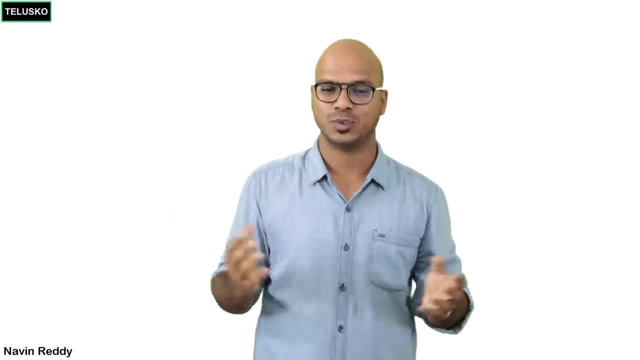 have to go back and then, when you come back, you have to again spend 30 minutes just to get into that zone. So scrum master will make sure that you have a meeting and then, when you come back, you have to have a meeting so that you don't have any distractions or unwanted meetings. But what? 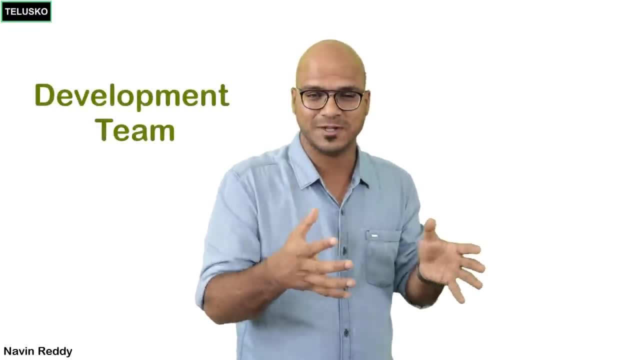 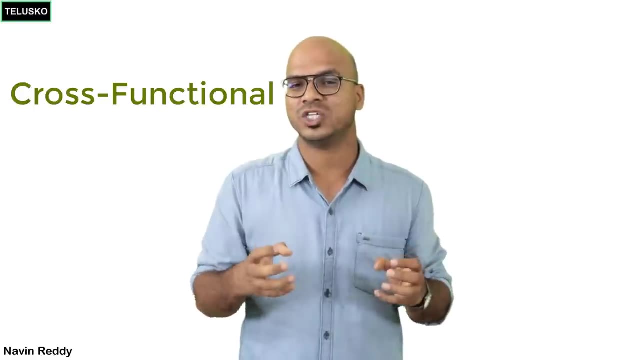 what about development team? do we really have? let's say, we have six people. do we really have one tester, one developer, one deployer? Not exactly. This is a cross-functional team. Basically, every person should know everything, So one person will know testing. the same person can be developer the. 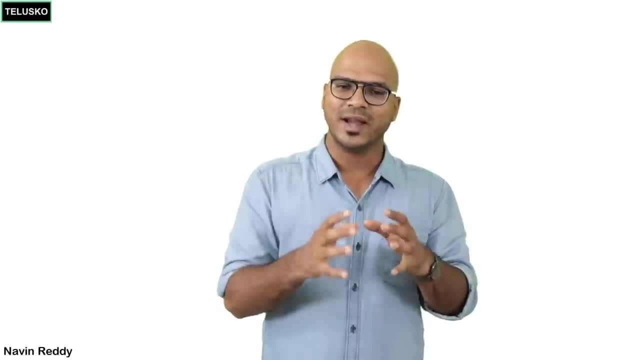 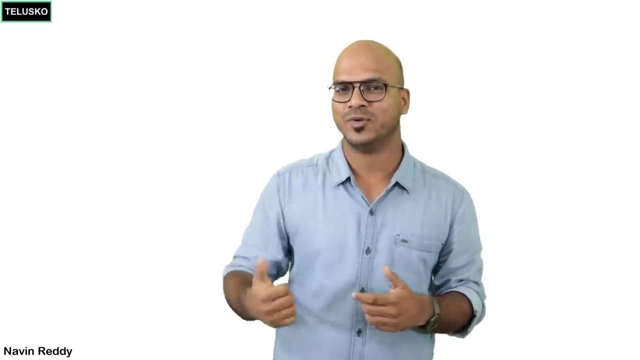 same person knows how to design a software right. The advantage is if you're not depending on someone else. if that person's not there in the office on that day, you should not say: we don't a tester, so we can't test the software. you can do it, so the development team is self-organizing. 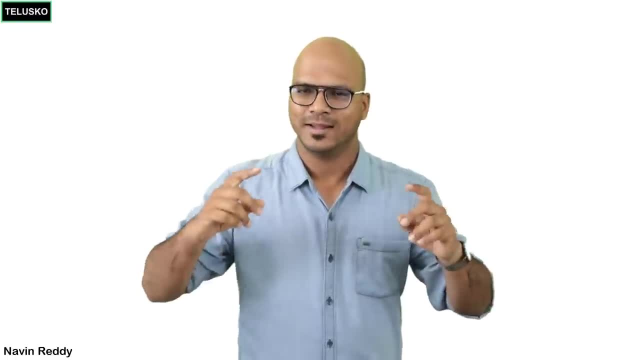 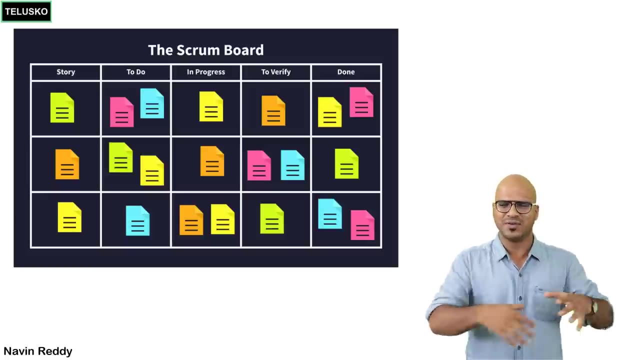 and cross-functional. now, how will you implement this? now, there's one important thing in scrum which is a scrum board. so basically, you know what is scrum board. so normally, when you work on your requirements, we have a team of six people, right? so you should know what is happening in the 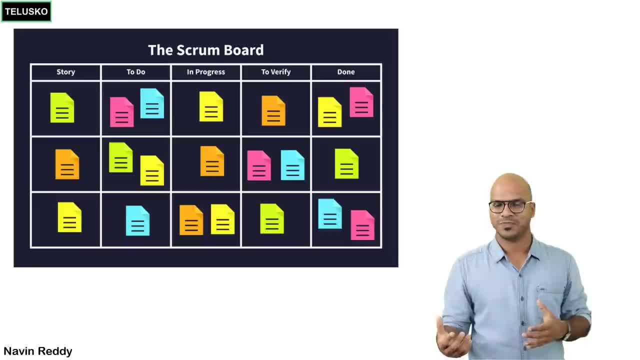 project. so there should be a clear picture. what is the progress? right? so let's say we have six people and they are working, so of course you have a sprint backlog there, so you can create a board something like this, where you have the first column, where you have the entire backlog. 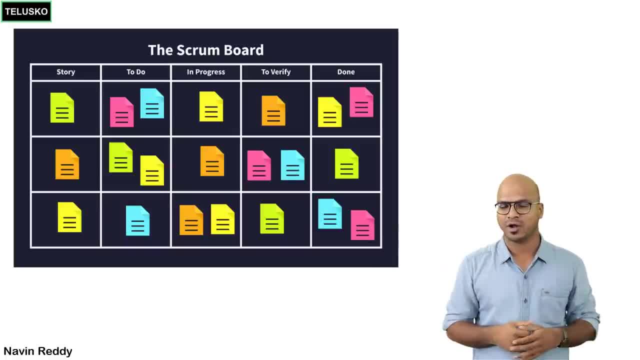 uh. then you can specify, uh, what you're currently working on, that is your 2d list, and then what is your current you're currently working on and what is done now. that is very important here. now, when you say done in in agile, it is, it should be done, done right. so there's a 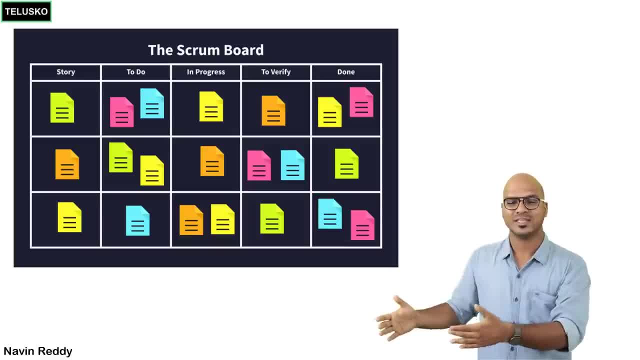 different definition for done. if the product is not working, it's not done okay. so you should not say it is 75 percent donation, it is not 80 percent done. when you say it is 100 done, then it is done okay. so that's something you can put in the last column. so basically, it is developed, it is 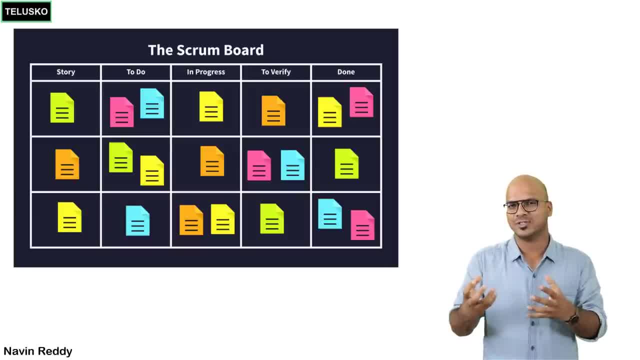 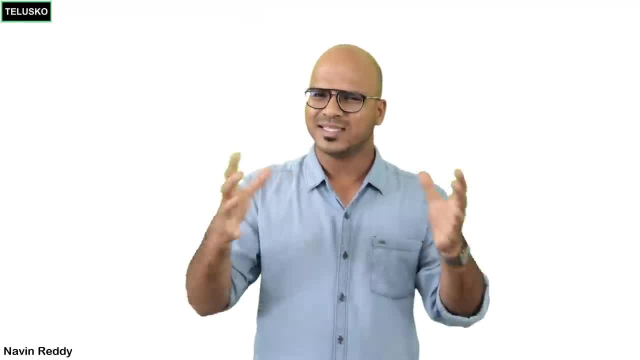 tested and it is rated for a shipment. so that is, that is your done definition, and if you can do that, you're basically following agile and you are working in this current framework. so, yeah, that's about this current framework. i hope you enjoyed this video. let me know in the comment section. 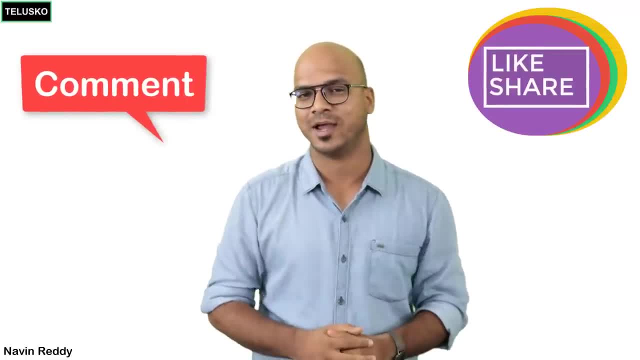 and do subscribe for the videos, because we'll be having amazing series coming up. bye everyone.